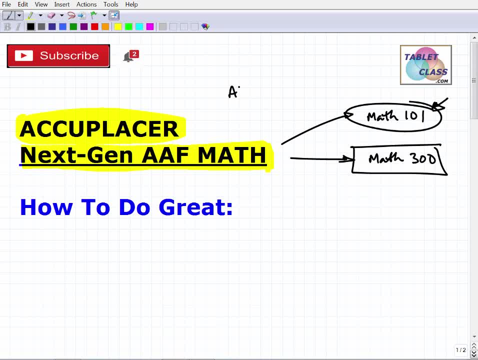 Okay, so you want to place into the highest level math class for your abilities. But I think a lot of students assume automatically: oh well, You know, in high school I took Algebra 1,, Algebra 2, pre-calculus. I did great in pre-calculus. I got A's in all my tests. 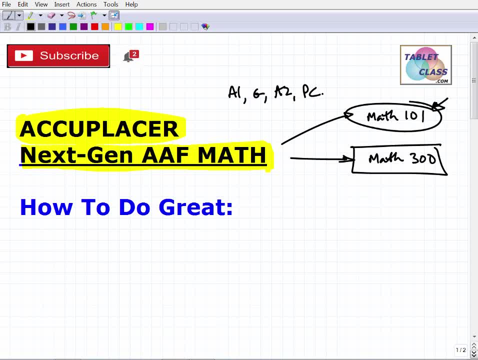 Hey, that's great, but guess what? That really doesn't mean anything when you take the ACCUPLACER, unless you do the following, And that's what we're going to talk about in this particular video. I'm just going to highlight some things you want to be thinking about when you take or you study for the ACCUPLACER: Next Generation AAF test. 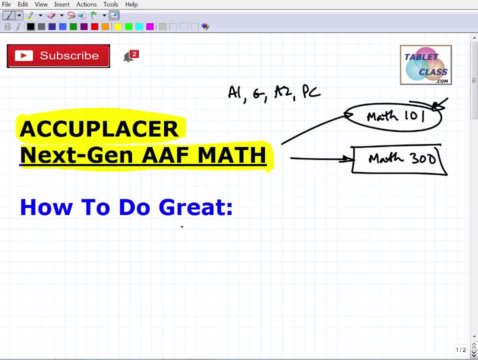 Now my background again. I'm a math teacher. I actually constructed a very good course for the Next Generation Advanced Algebra Functions- ACCUPLACER. I'm going to leave the link to that course in the description of this video. You can check it out if you like. 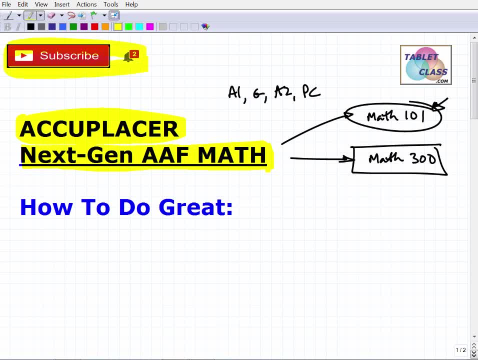 Also, I literally have hundreds of videos that can help you prepare for the ACCUPLACER- all the various ACCUPLACERS, in terms of the mathematics. So hopefully you'll consider subscribing to my channel. But with that being said, let's get into this video. 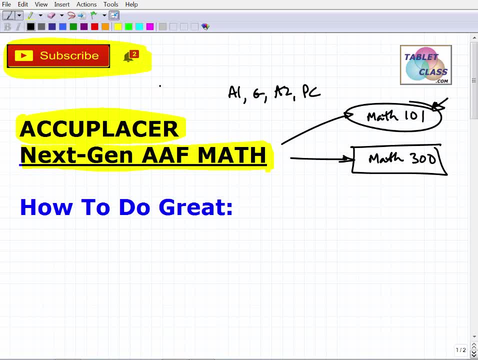 So how do you do great on The ACCUPLACER Next Gen Advanced Algebra Functions test? Now, first of all you've got to respect the title. OK, advanced algebra and functions, OK. so advanced algebra means it's more than just algebra one. 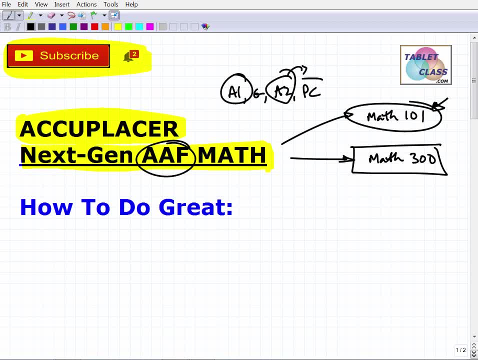 OK, it means for sure, algebra two and definitely concepts. algebra concepts into pre algebra- OK, I'm sorry, pre calculus. So you know these are fairly sophisticated topics. So you've got to know your stuff and, trust me as a teacher, there's plenty of students who can get good grades in their class because they're taking a test. 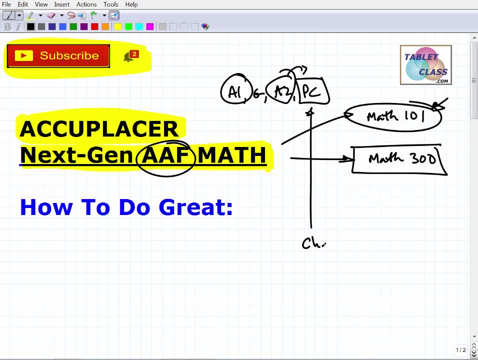 Let's take pre calculus, right, They're taking a test, one chapter at a time, typically, So this chapter. all they're focused on here is, let's say, systems of equations. OK, so they're focused only on systems. 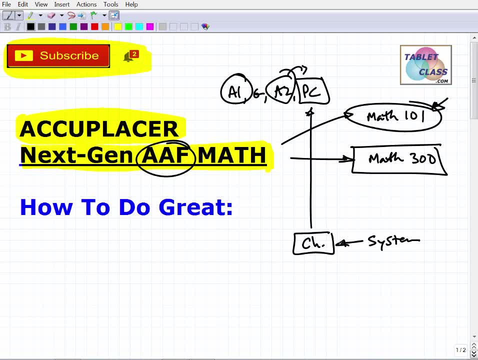 They're going to take a test on on on this chapter And they do Well, they get 95 percent and they're happy with it. And then they move on to the next concept being taught. Let's say maybe it's, oh, quadratic functions, or whatever the case might be. 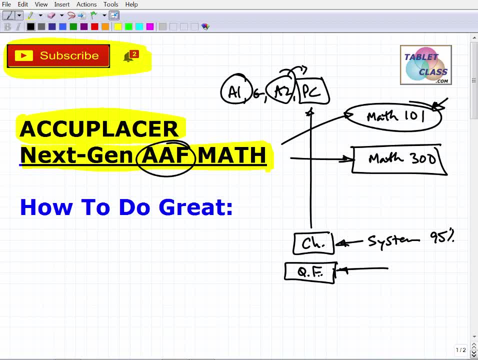 And the same thing applies. You're studying kind of, I would say, in a vacuum, but you're studying only specifically for that one chapter at a time. Now, this ACCUPLACER, it's a placement assessment. Well, you've got to be, you know, thinking about all of this. 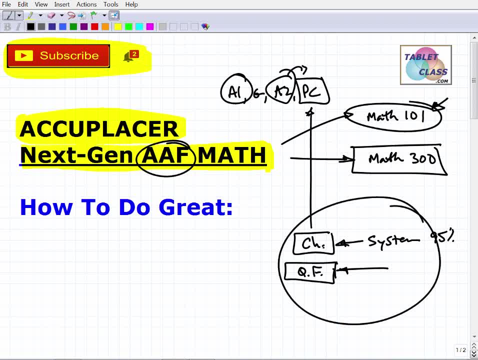 All right. So just because you're you're a good test taker And I don't want to diminish that, by the way. if you're able to do well in these tests, that's definitely good. You know very good. 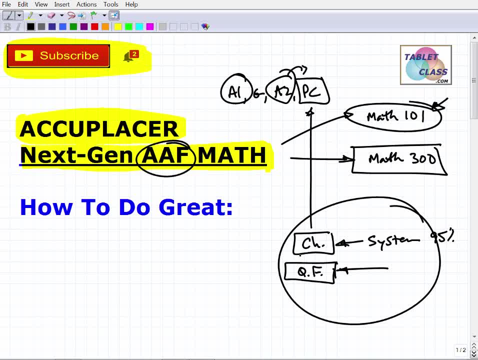 But it's your ability to retain. OK, retention, true retention of this material only comes through mostly if you really understand it, And that sounds kind of like obvious. But if you really understand something you're going to retain it And I've seen plenty of students who've been able to kind of test well, but they didn't really kind of understand it. 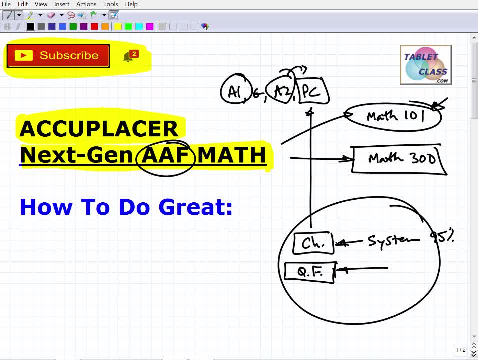 They just studied really hard and just use a lot, You know, muscle memory and rote memorization flashcards just to do whatever they can to get a good grade. And that's respectable as well. But that's not going to be as beneficial to you, for sure, on a test or an assessment like the ACCUPLACER. 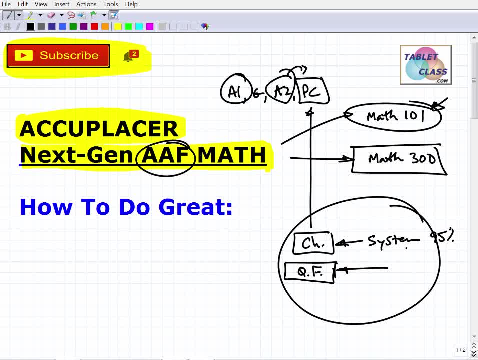 OK. so again, if that's your kind of your style of studying, where you, like you know, go through with a bunch of flashcards and stuff, you know you want to try to move away from that and focus on true understanding. 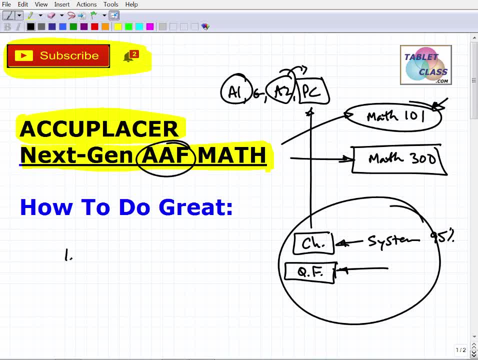 So the first thing I would want to do is: you know you're going to have to be a good test taker, So the first thing I would want you to kind of think about when you're studying for the ACCUPLACER AAF is to review, obviously. 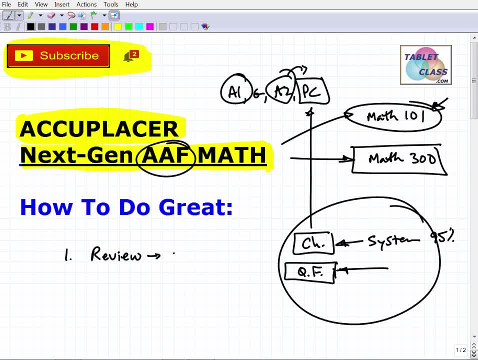 but review with the kind of the spirit or the intention of truly understanding- OK, understanding, not to review for review's sake, And that's kind of a fine line. You're like, oh yeah, I can be reviewing, going through my notes and all this other stuff just to kind of brush up and try to brush up on my memory. 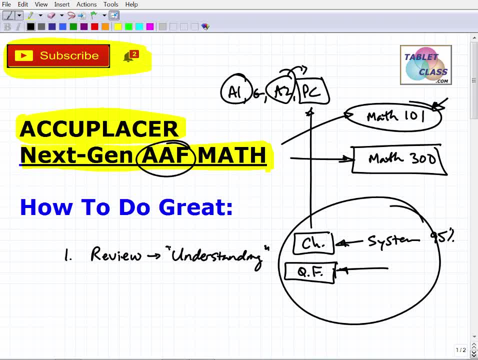 in terms of the math, And that's kind of a fine line. And that's kind of a fine line. But try to look at math in a sense that, hey, I need to really kind of understand this, this, this skill. 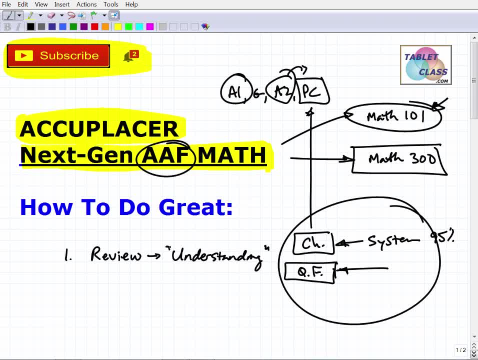 You know I need to understand this concept, OK, because if you can do that, that's going to not only serve you well on the ACCUPLACER, but you know future math courses as well, And so if you're going to be doing the advanced algebra function assessment here, chances are you're going to. you know. 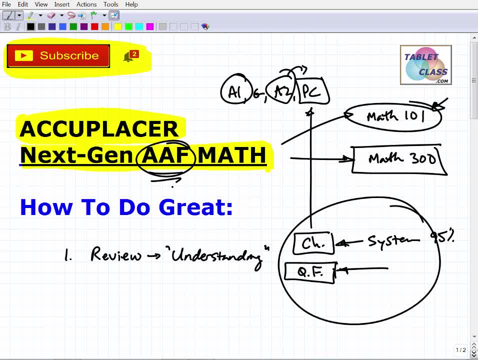 be taking some pretty sophisticated math In college, right, Probably many of you are going to be going on to calculus and you- just you know it's very difficult to try to do well, let's say, in a course like calculus, by just you know, using flashcards or without really kind of understanding the concepts, is. it's kind of what I'm getting at. 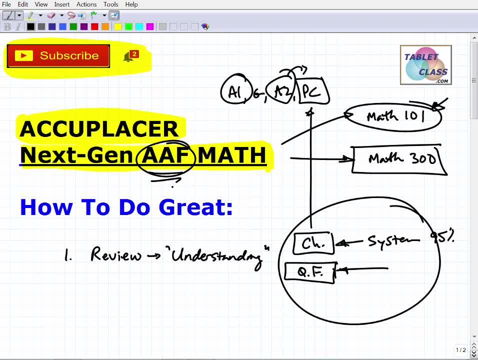 So if you were that student in high school that you know just kind of like looked at math as OK, I'm just going to just, you know, do what I got to do real quick just to do well on a test. 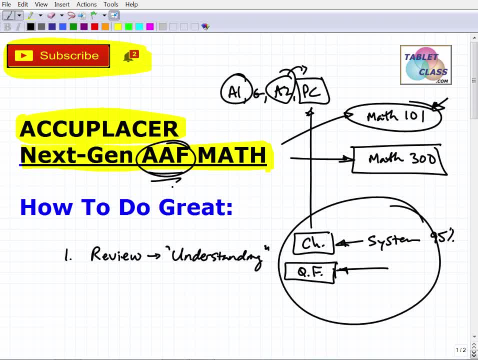 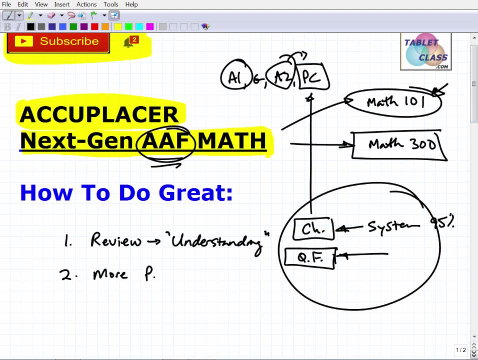 Well, try to change your philosophy, again in terms of: All right, let me really try to understand this stuff. OK, All right. So the second thing that I would kind of stress- and this again it might be kind of obvious to you- is really more practice, more practice problems. 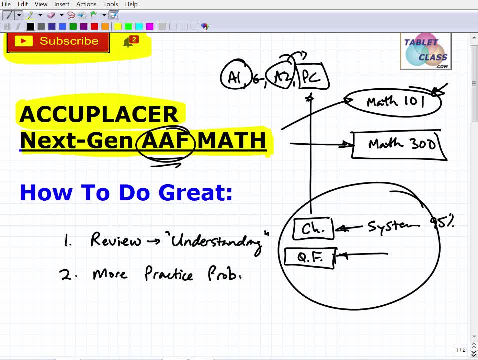 OK, Now what do I mean by that? Well, let's take a concept. let's say, like systems, just because you do, you can do a few systems problems. you practice, you know. OK, I can solve this problem. I can solve this problem. 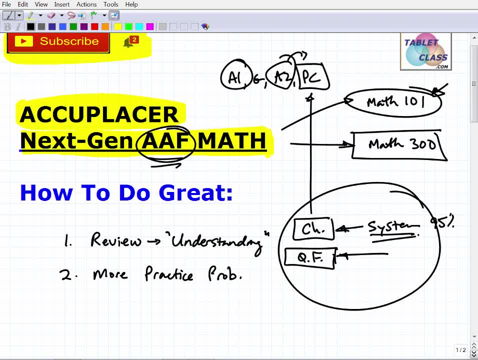 That's not general. It's not only indicative enough of like your readiness for that particular skill. OK, You really need to challenge yourself with a lot more variety. you know of problems to really feel good about. you know your understanding of particular math skill. 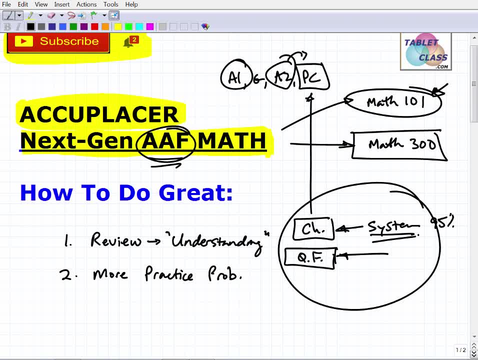 OK, A lot of students kind of get this self, what's it with this kind of false sense of security? But say, OK, let me see I could do this problem. They might not even do the problem, They'll look at a problem. 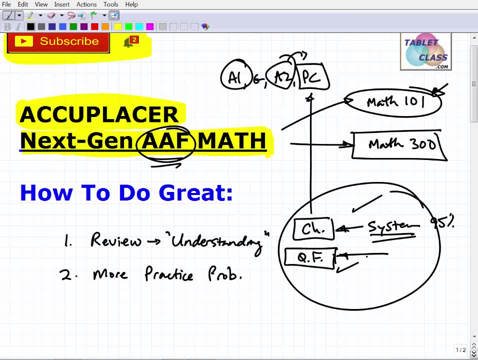 They'll say: oh yeah, I know how to do that, I know how to do this, But they haven't even tested their ability to actually check their understanding. But I'm going to tell you right now: math is a skill. 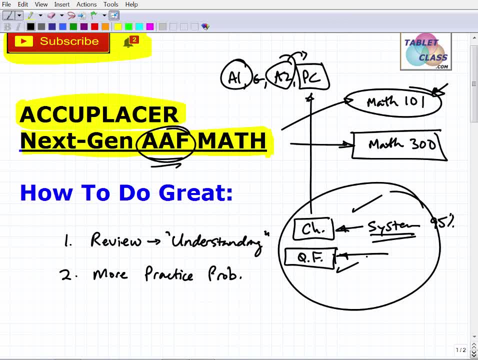 It's a language as well, And the only way you get good at, let's say, speaking Spanish, or you know any skill playing a guitar- is to do it a lot. OK, You need to do a lot of math practice. 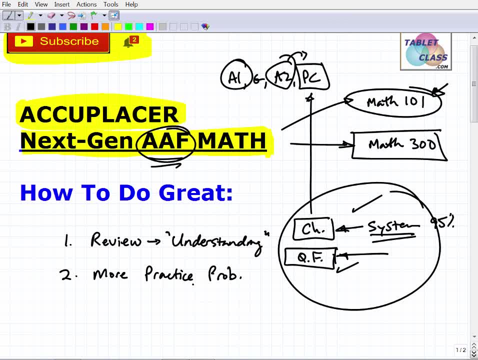 But before you go practice, OK, you need to kind of learn and review. That's what I've done in my particular course, my Accuplacer, Advanced Math. So I've done a lot of math. I've done a lot of math. 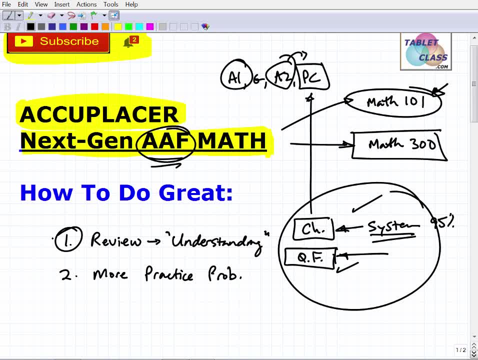 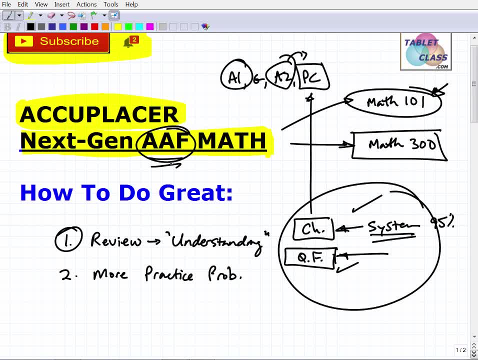 And I keep revising and improving these courses. But 23 chapters- no way you're going to be able to learn all 23 chapters. You have to go in and basically assess: hey, what do you know and what don't you know? 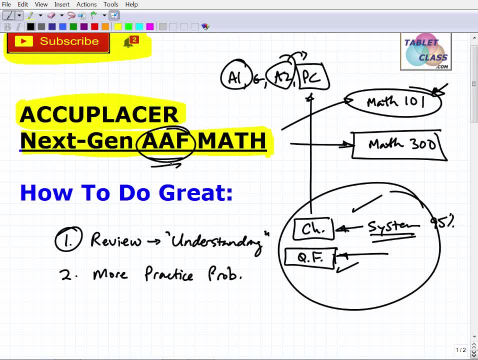 OK, So you've got to really think this stuff through. OK, you've got to get yourself organized. but if you have a good, organized, efficient plan, you don't have to try to relearn everything you're studying in high school, because that's just not practical. You can't take each one of these books. 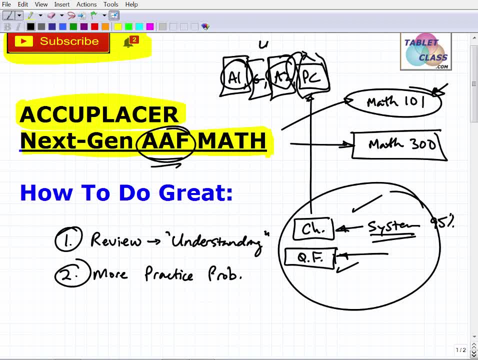 these textbooks and then reconstruct, let's say, four years of learning in four weeks or four months. It's not practical. However, what you need to do is to assess what you know, what you don't know, and then have a logical approach. But again, is it worth? 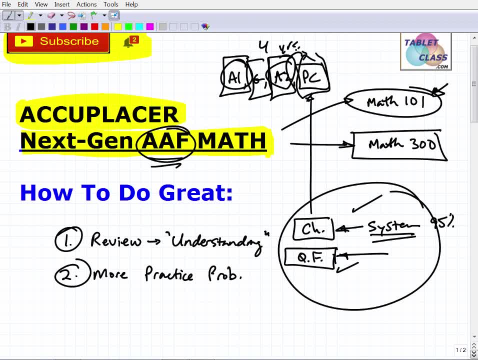 doing all this? Is it just easier just to take the ACCUPLACER and just do a quick review and then hopefully you kind of land into the right course? Yeah, you might get lucky enough to do that. but either way you slice it, you're going to need your math skills. 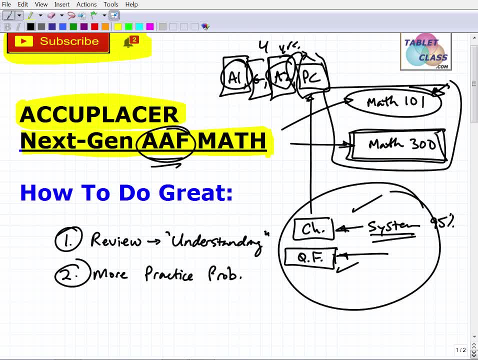 Let's say you do land into the higher level math course. You don't want to be that person that comes into it unprepared, Like you just minimally got into the course and now the teacher's like, okay, hey, we're right off to the. you know we're doing. 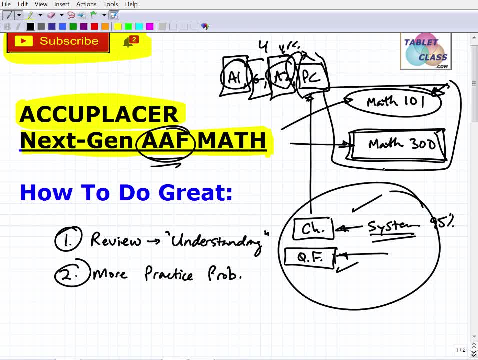 pretty advanced math because the expectation, especially in college, is you're already coming in the door with these math skills. It's not like high school where the teacher will spend some time reviewing, assuming that student's kind of forgot a lot of material In college. 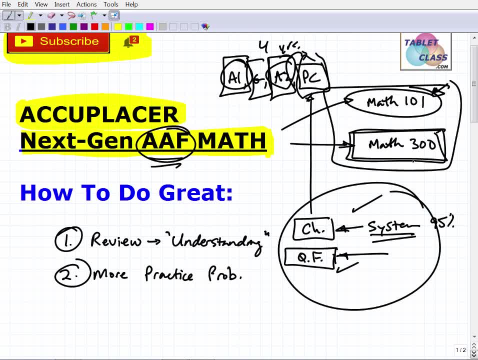 it's like, hey, we're moving forward, You're supposed to come in the door with this material. So in some ways, if you're not ready, you're better off going into, you know, a lower level class, just to kind of bolster up and strengthen. 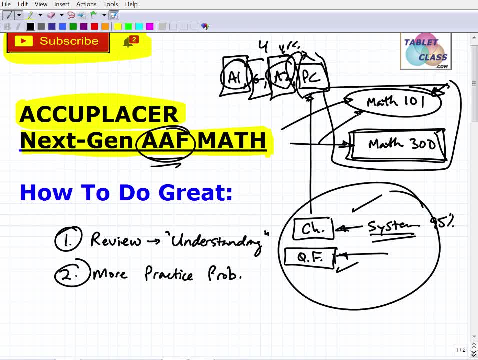 your material. But again, I think the whole purpose of this video is just to respect the level of math that's going to be on this particular ACCUPLACER okay, and really approach it with the spirit of you know, understanding, okay, math for what it actually is, not just 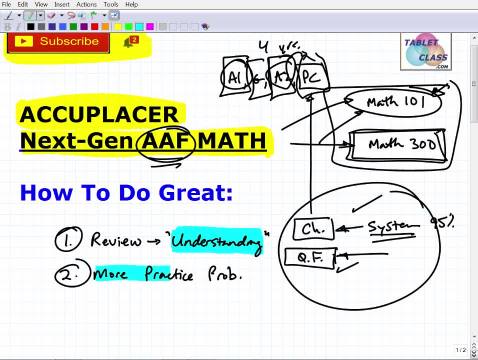 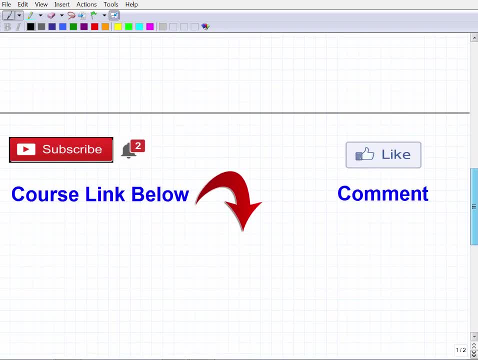 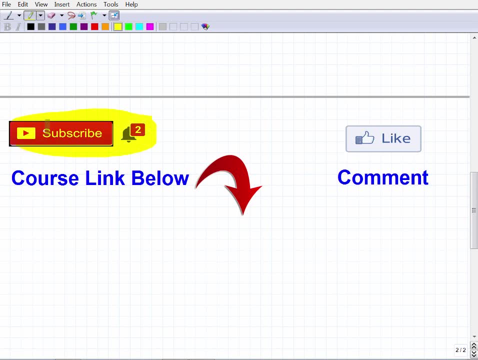 passing the test, if you will. And again, the more practice problems you can do, the better off you're going to be. So let's go ahead and wrap this video up. And one more time. you know, if you like my teaching style- and you can check out a lot of my videos again on my YouTube channel- 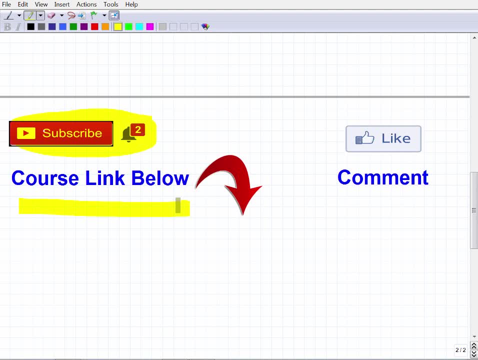 but if you want to just check out my course, my ACCUPLACER Next Generation Advanced Maths and Functions course, I'll leave a link in the description of this video. You can check that out if you like. If you enjoyed this video, I would appreciate a thumbs up and. 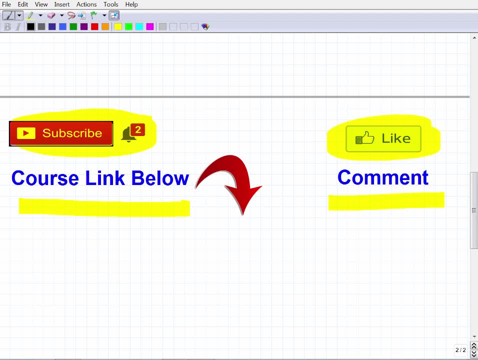 leave me some feedback. Let me know if you're you know taking this, you know this course, or taking this ACCUPLACER for the first time or the second time, or maybe you're taking another placement exam. There's other ones out there, like Alex, for example. They're. 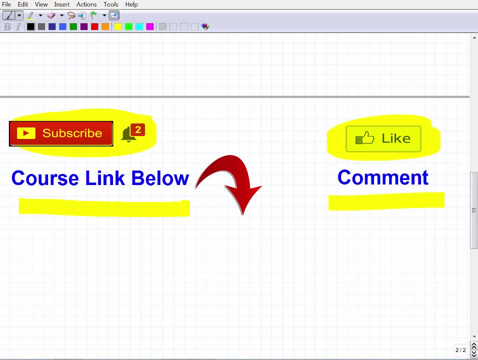 all good, but they are kind of different in various ways. And then there's other things out there, like the CLEP exam that some of you may have heard of as well, where you, instead of placing into a particular course, you can test out and get credits for what you know. 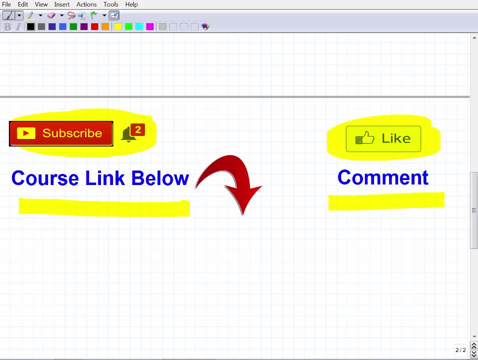 That's a great program as well. So a lot of things, A lot of things that you need to kind of be, you know, informed about. if you're- which I'm assuming, if you're watching this video, you're probably entering into college. you. 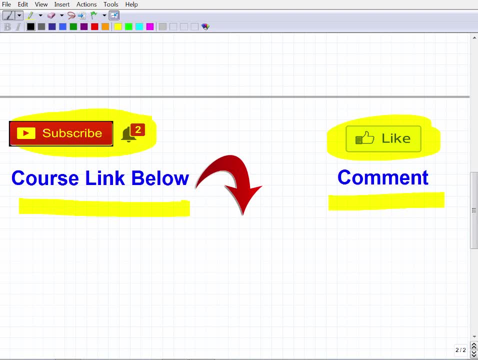 know your first year of college, So there's a lot of different options and opportunities out there, but hopefully this video helps you out. So, with that being said, thank you for your time and have a great day.